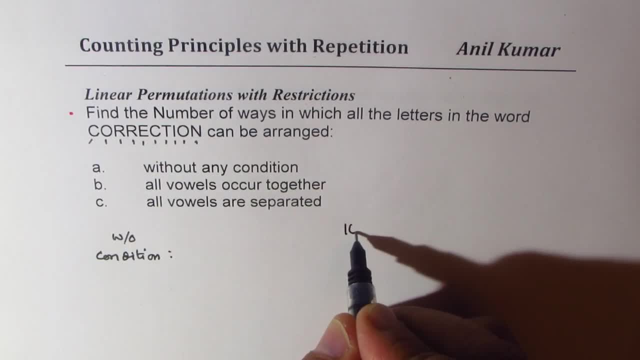 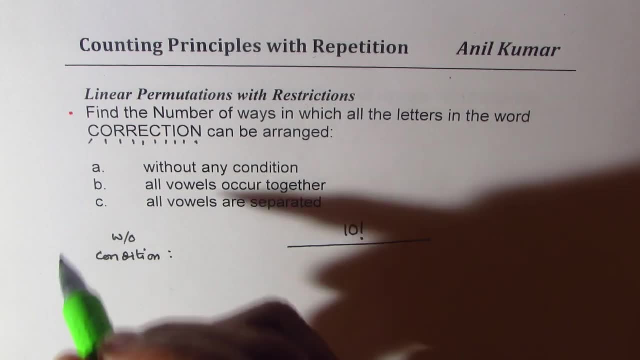 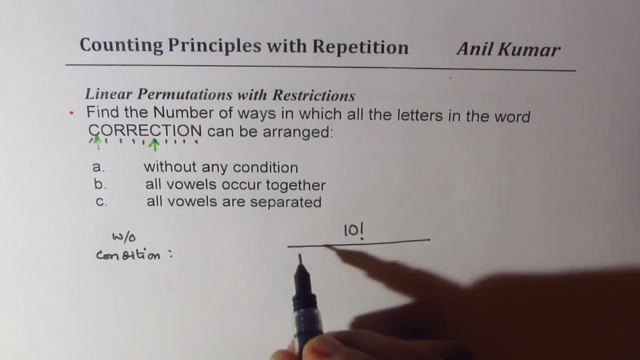 The number of ways will be- since there are 10, it will be 10 factorial divided by how many are repeated. Let's see. So we have two C's here, So there are two C's. So that means, divided by two, factorial for the C's. What else, As far as O's are concerned, 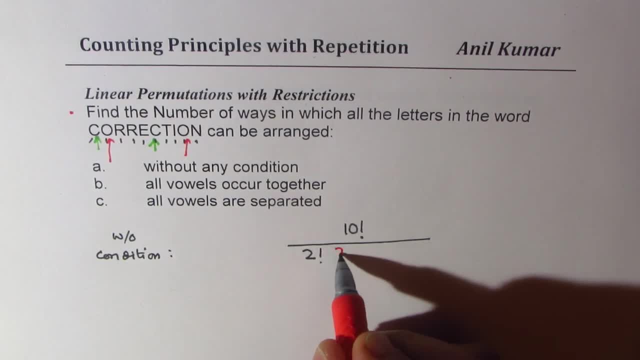 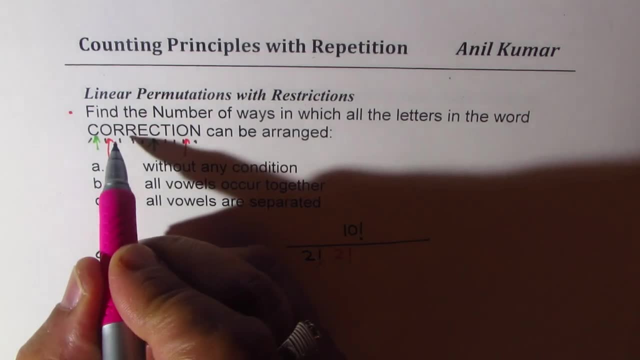 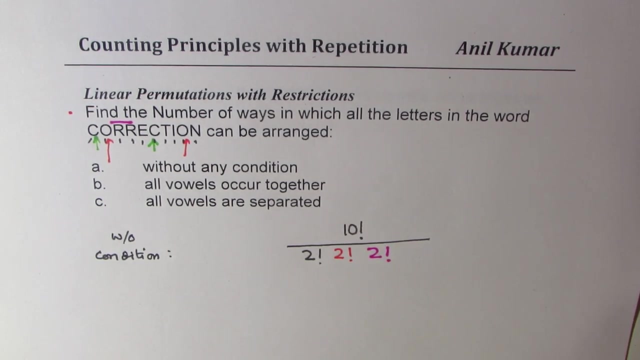 we have two O's also, So we'll divide by two factorial for O's and we see those R's together. Two R's also, So divide by two factorial. So whatever is repeated, since those words form, With or without meaning, will be exactly same. so we have to divide by those numbers. 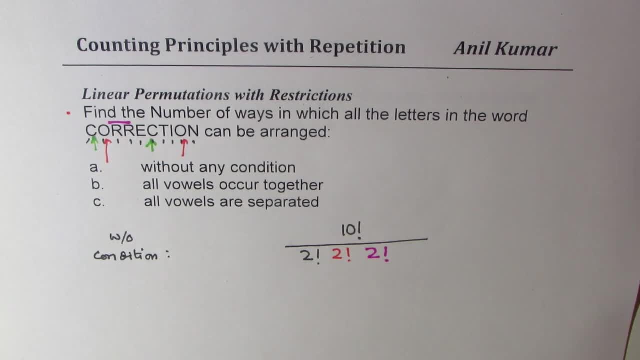 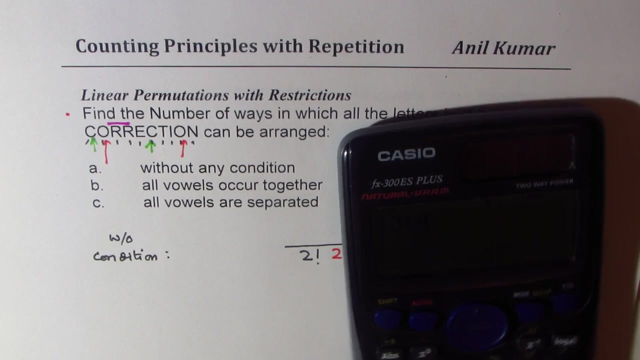 so that gives you the answer right. so 10 factorial divided by 2 factorial divided by 2 factorial. so let's take a calculator and Find the exact value. So we have 10 factorial Divided by. we can divide by 2: 2. 2 means 8. 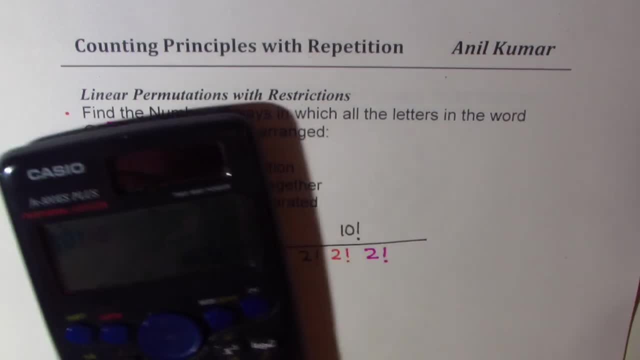 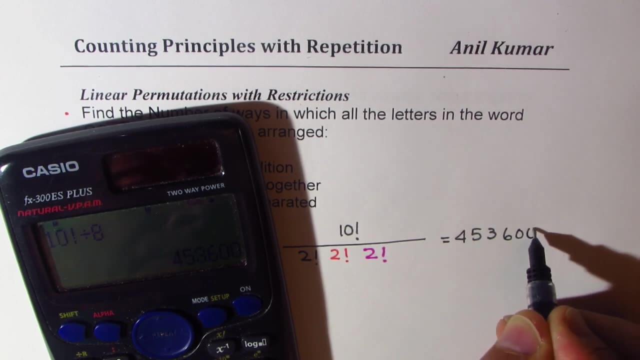 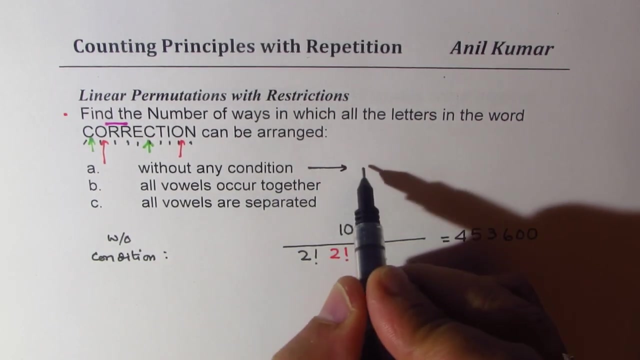 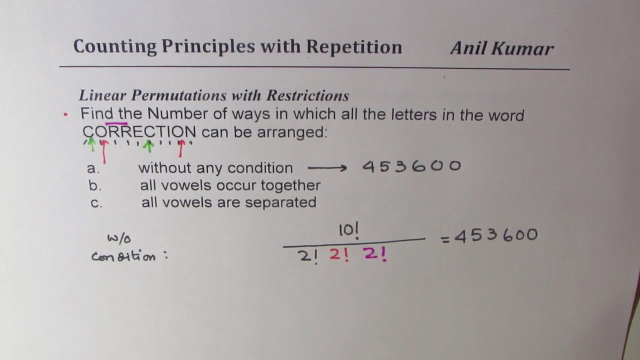 Let's me just divide by 8 and what we get is a very big number, which is 453 600. So these are the total number of ways without conditions. so the answer for the first one is 453 600. So I hope this is absolutely clear. now Let's see when we have conditions, like all. 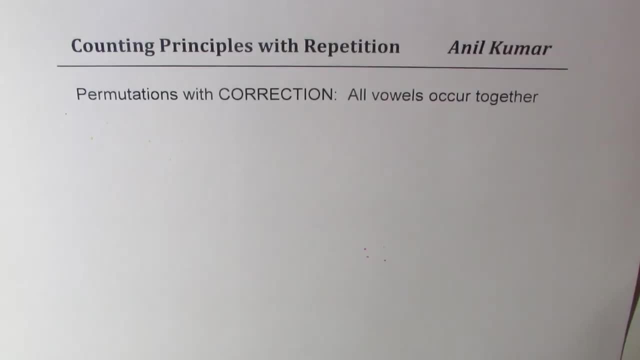 Vowels occur together. How can we do it right? so let's again take up the same question. the word here is Correction, so let me write down the word correction and then we'll look into all the vowels. So the word is C O. 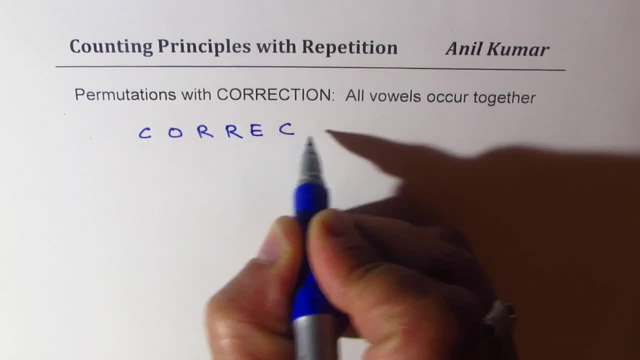 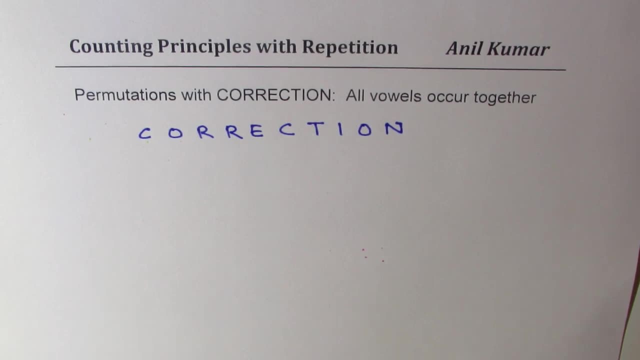 R R E C T I O N. Now, what are the vowels in this? A, E, I, O, U, right, so we have I O, so we have these four vowels. Now, in this world, let's write down what all we have, and then we'll figure out the answer. so, as you can see from here, 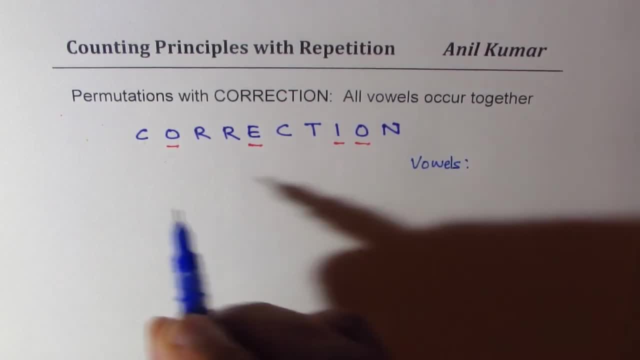 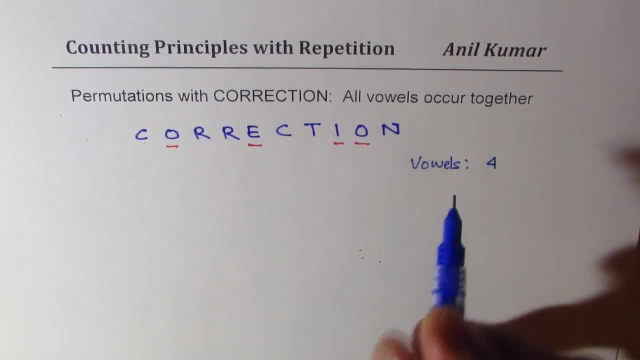 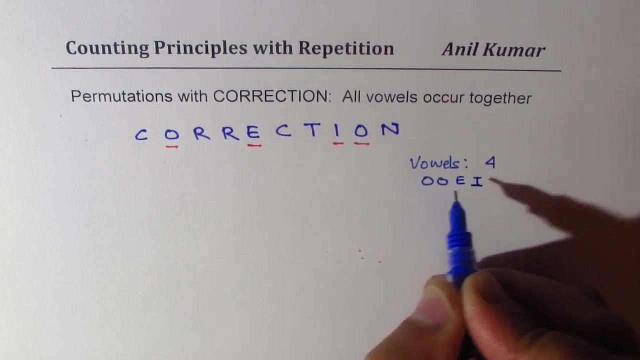 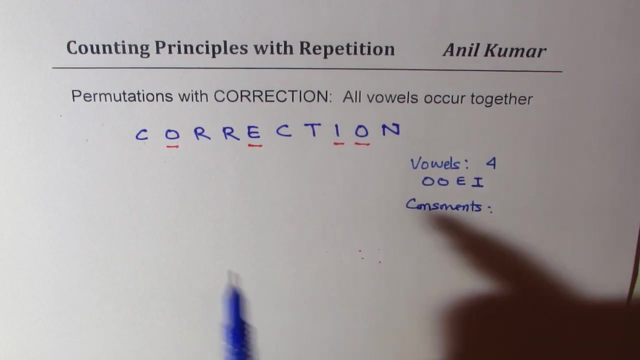 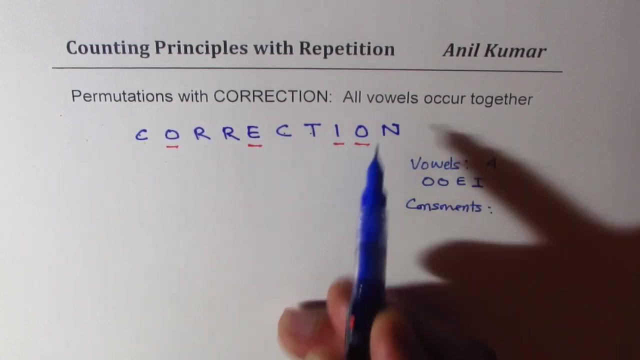 vowels are four and These vowels are O, E, I, O. Right, so these are. let me write O's together: O, O, E and I. So these are the four walls, So a consonant. Consonants are total number of words Which we saw at ten, one, two less. count them like this: one, two, three, four, five and one six. 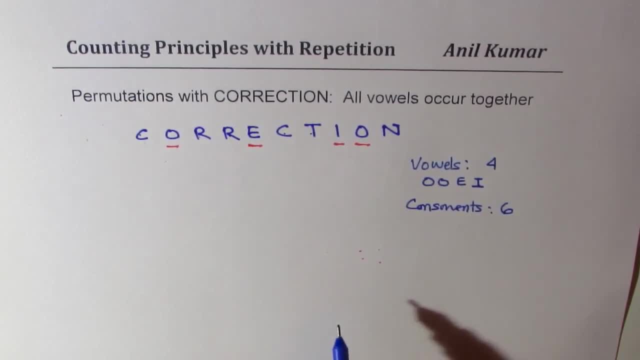 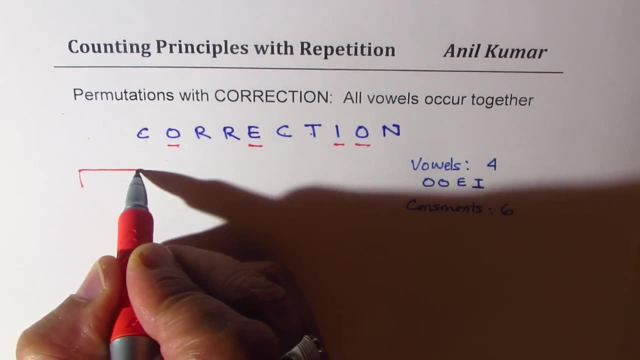 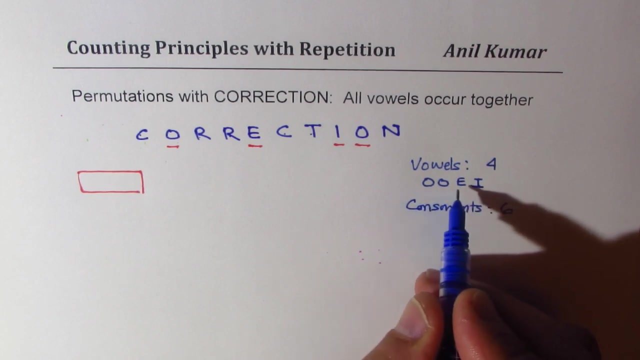 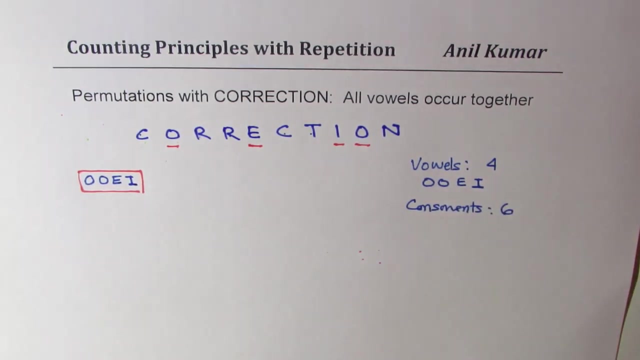 ten minus four. those, those are the consonants. now, when we want to put all the vowels together, we can actually form a group, and in this group we can place all these vowels. so which are oo ei, so it is oo ei. so once you place them together, then we are left. 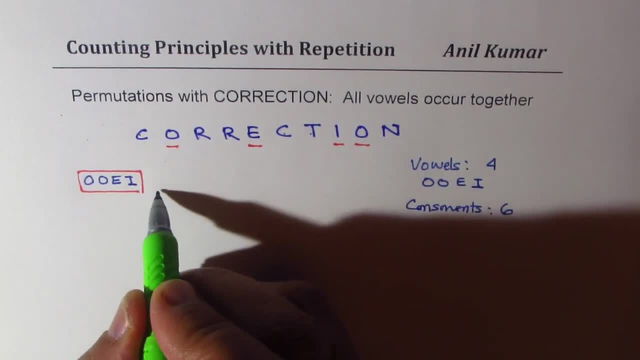 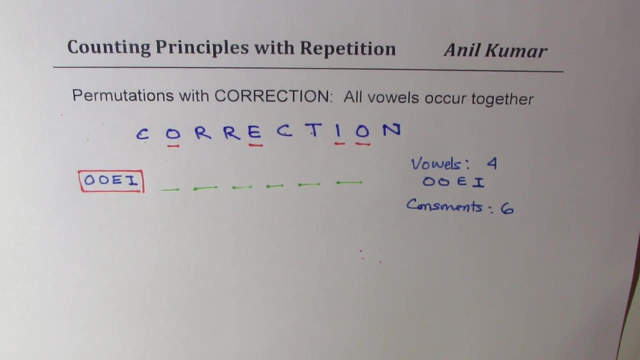 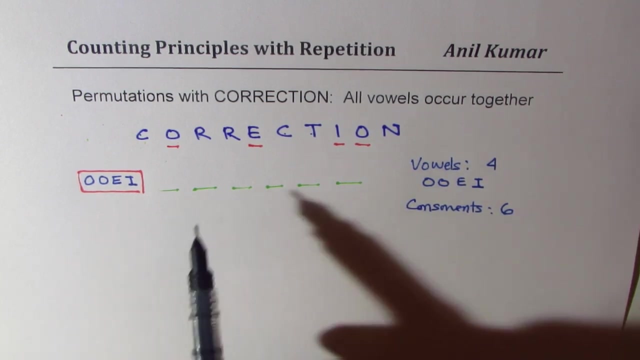 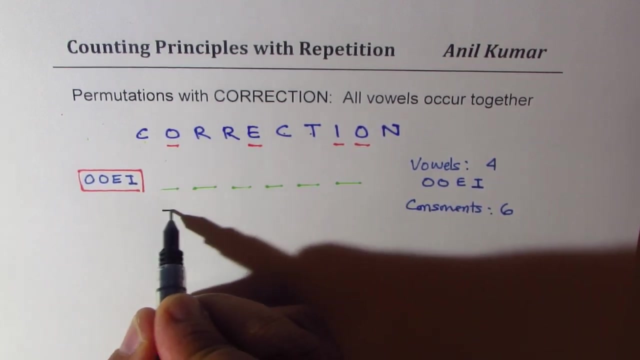 with how many positions? we are left with six of the positions: one, two, three, four, five and six. now looking into counting principles, how many ways can you arrange these? so basically treat this as one letter, right? so it is one, two, three, four, five, six and one, seven. so we have seven factorial divided by all of these. 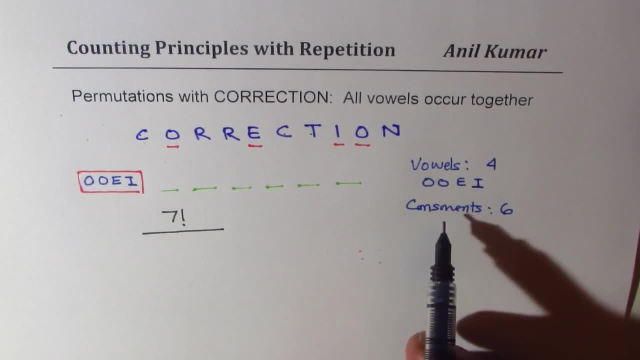 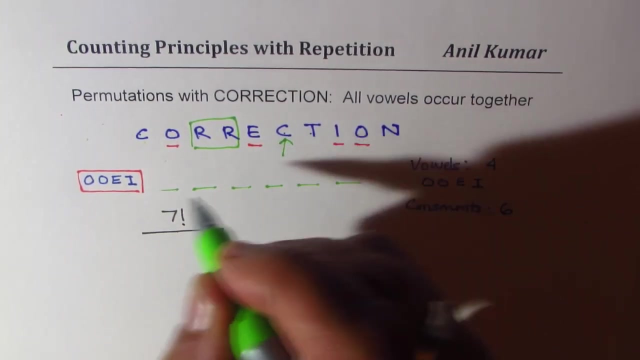 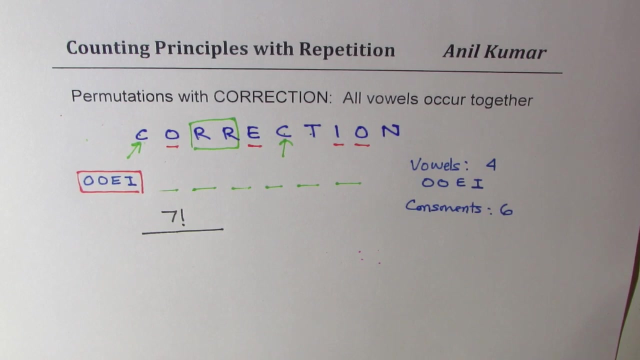 consonants. how many of them are repeating? right, so this is what we have to see. so, as you can note, here the repetition is because of ours, they are repeating and also because of C's, so two of them repeat to two times. so we'll divide by two factorial. 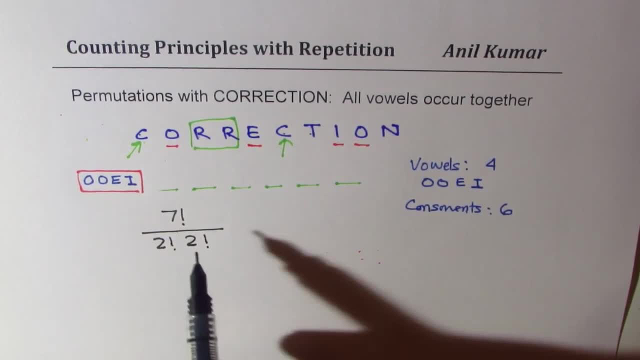 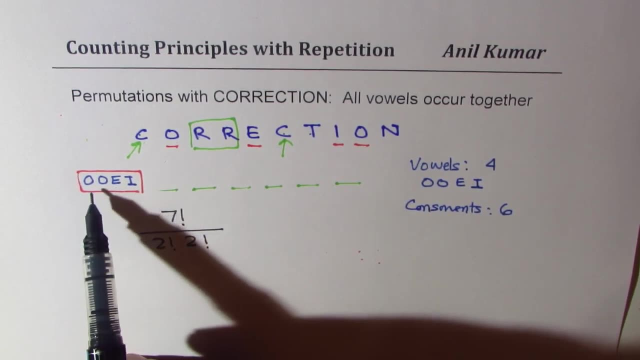 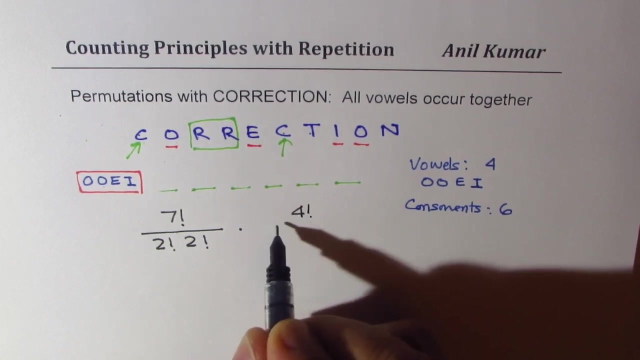 right. so these are the ways in which all of them can be arranged. now, for all these combinations, we have these four vowels. they can be arranged separately, also right? so since there are four, the ways in which you can arrange these vowels are four: factorial, divided by O's. repeat so over two factorial, you get an insight. 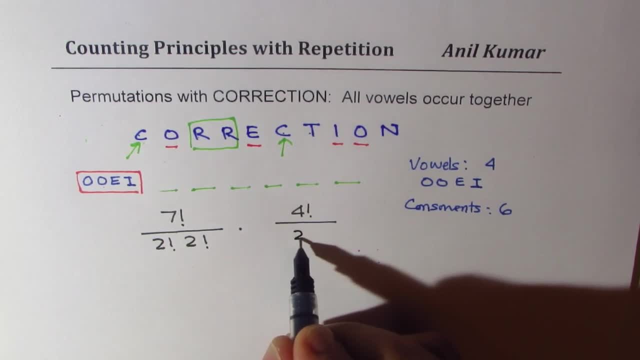 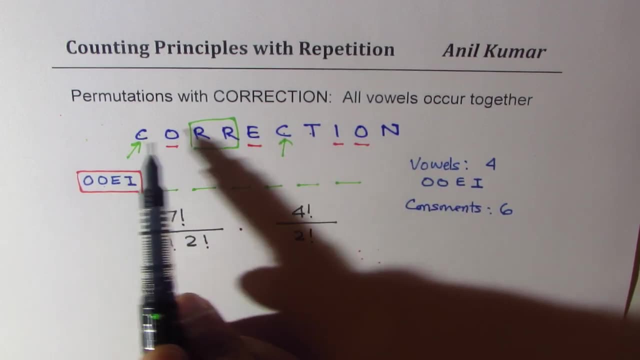 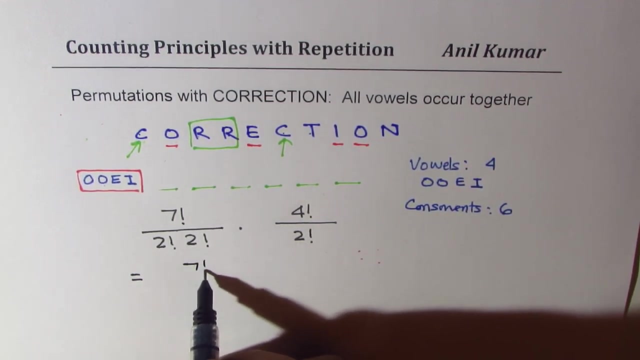 and the answer to this we need is the number of vowels. we have these four variables idea, so that becomes the solution, right. so permutations, with correction, all vowels being together will be equal to seven factorial times well. four factorials four times well. we'll do use calculator, so we'll not over. let's write this as eight. let's calculate this now. 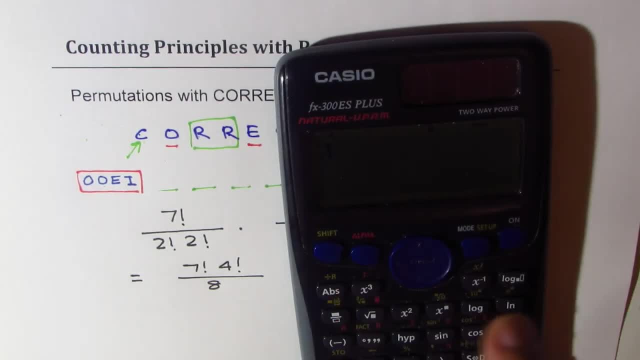 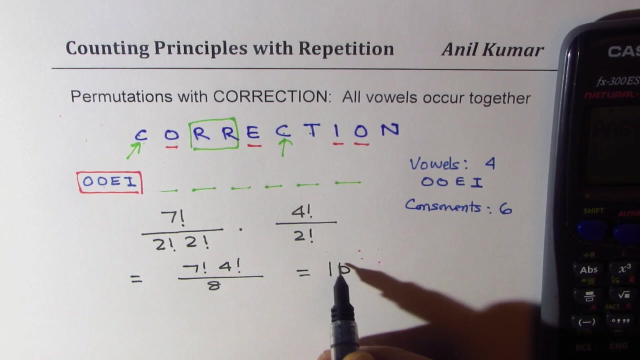 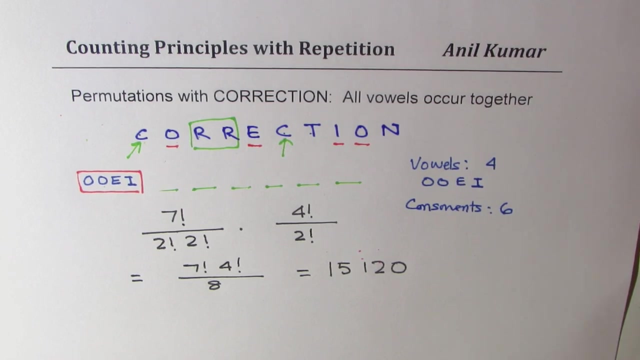 so we have seven factorial times, four factorial, and we'll divide this by- uh, eight, right? we get 15, 120, correct? so that becomes the answer for all vowels occurring together. is that clear now? the last part here is that we have seven factorial times, four factorial, and we'll divide this by eight, right? 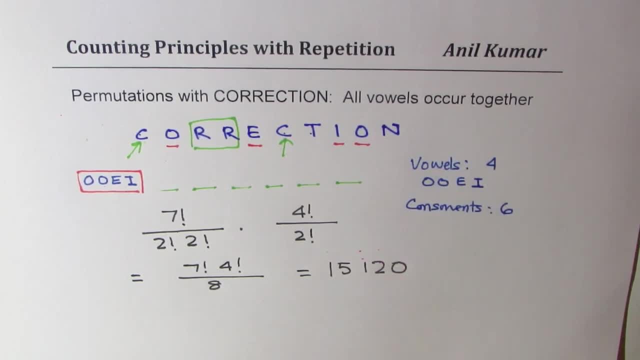 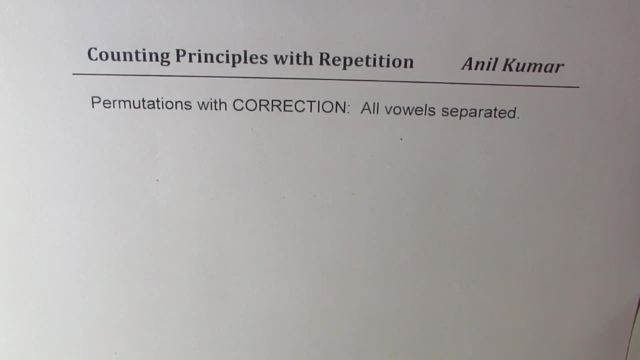 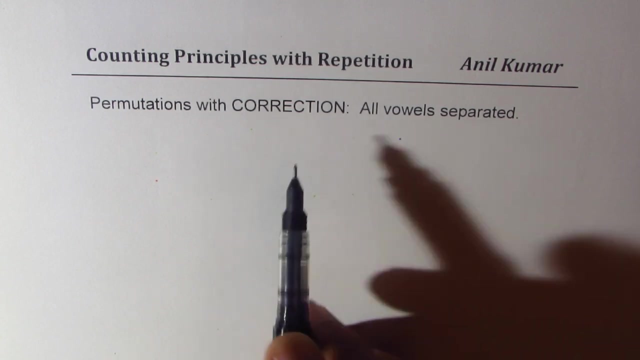 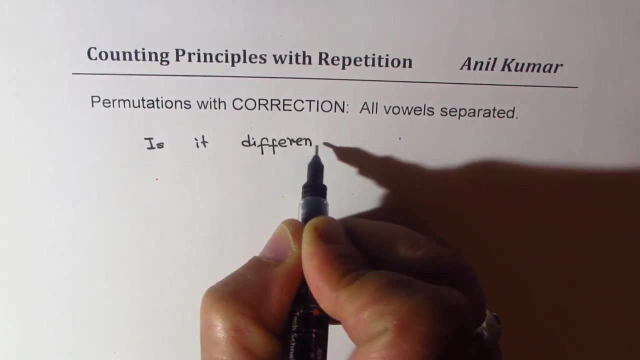 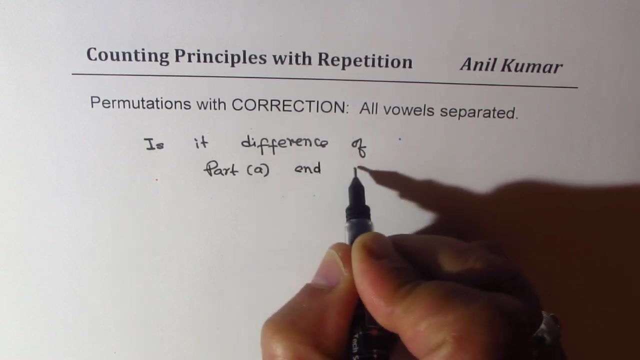 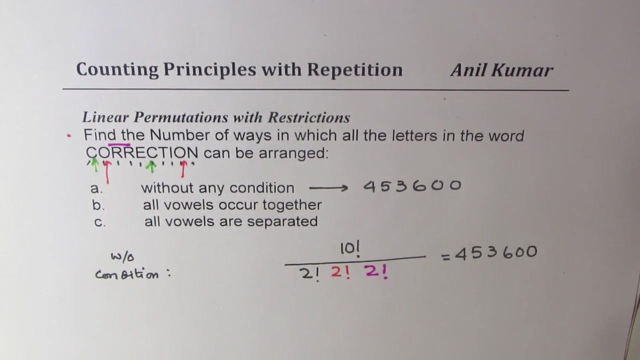 is when all vowels are separated. now my question to you is, when we are trying to answer this question: permutation with correction, all vowels being separated, can it be the difference of part a and b? so let me write: is it difference of part a and part b? well, remember, part a, for us, is without any condition and part b is all vowels occur. 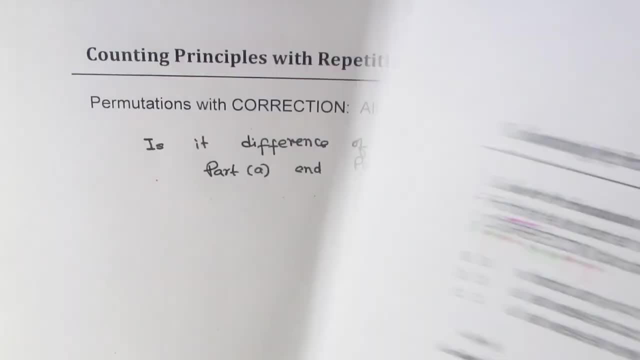 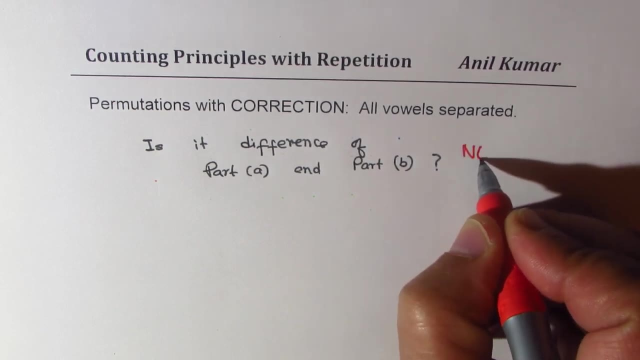 together. part c is: all vowels are separated. so that is the question first. you should answer. well, the clear answer is no, it is not the same. since we want the vowels to be totally separated, that means we want all vowels to be totally separated. so we want the vowels to be completely. 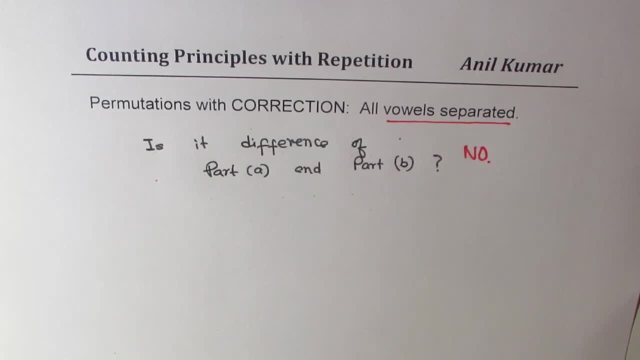 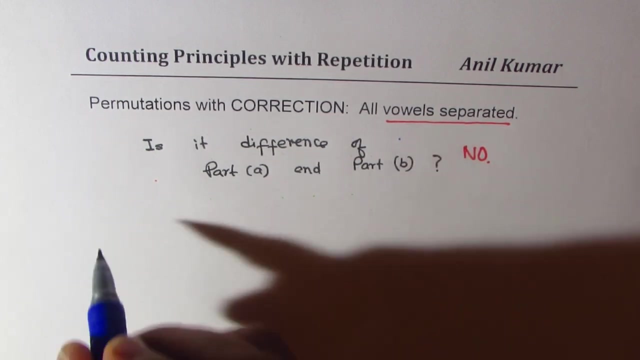 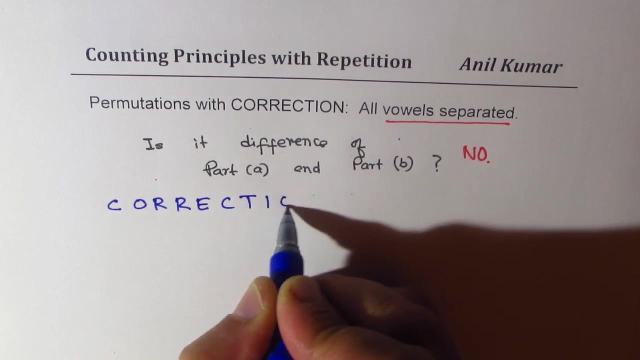 even two vowels cannot come together, right, or three cannot come together. if we do the difference, then all four are not coming together. so that is how they are different, correct? so let's analyze the word correction once again and answer this question. so word before us is correction c-o-r-r-e-c-t-i-o-n. now in this word we want all vowels separated. 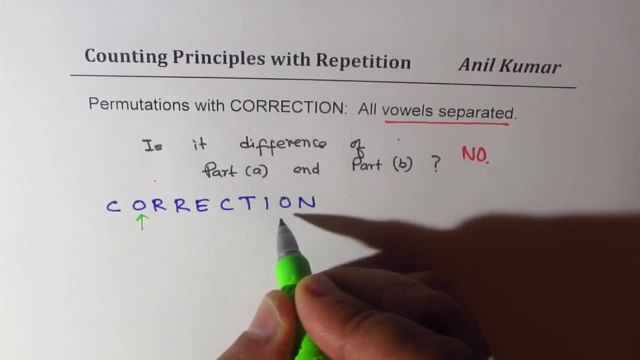 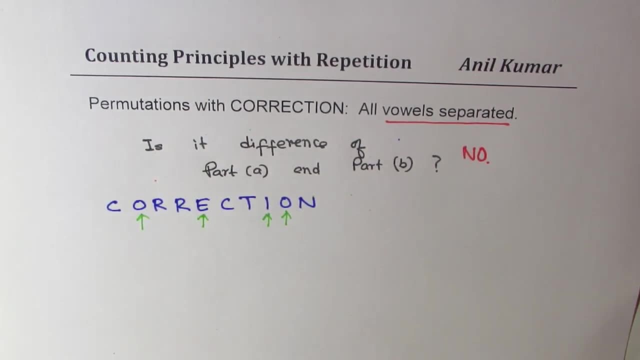 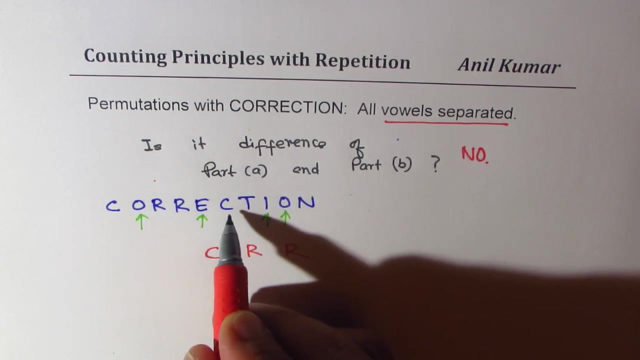 now, what are the vowels here? we have o-o-i-n-e, so these are the four vowels. so let's look into the words other than vowels. okay, so the words other than vowels are the consonants which are right on c-r-r, and then we again have c, then we have t and n. 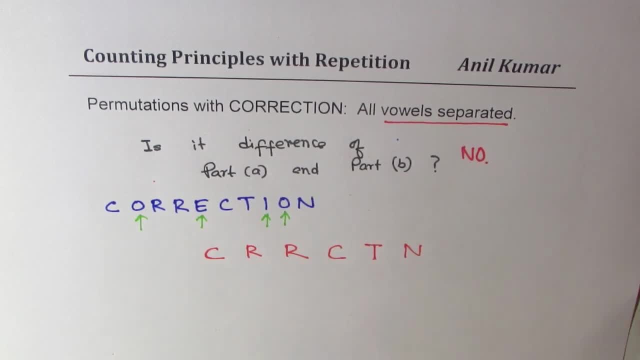 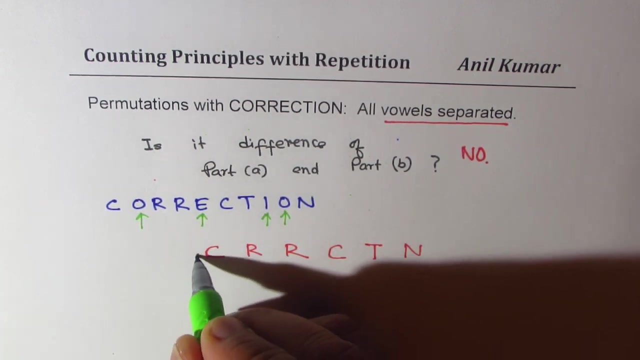 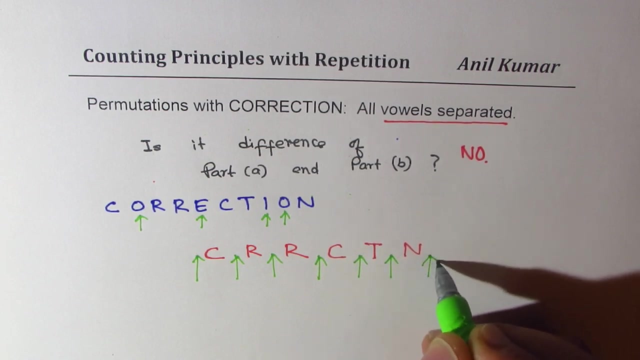 so these are the four vowels. so let's look into the words other than vowels: one, two, three, four, five, six of them correct. when we say vowels are separated, that means these consonants come in between perfect. so what could happen? these four could actually fill the gaps. we could start here. we could put one there, one there, one there or different places, right? so 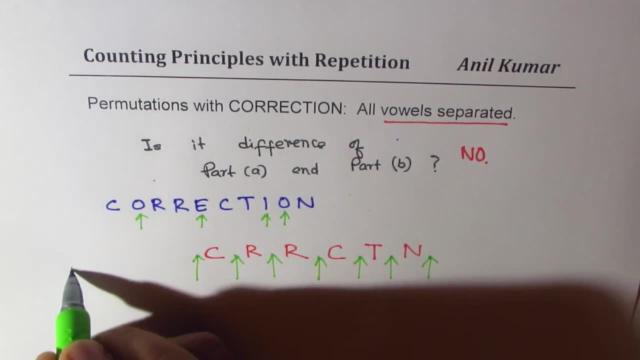 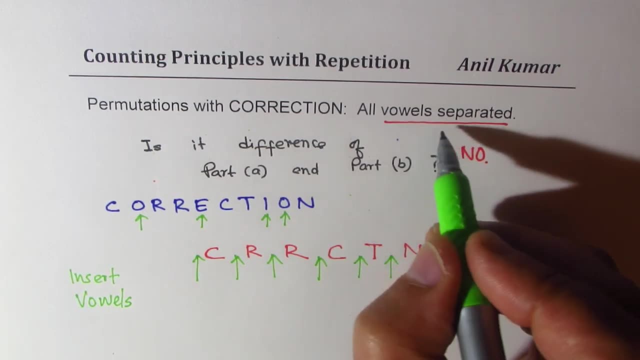 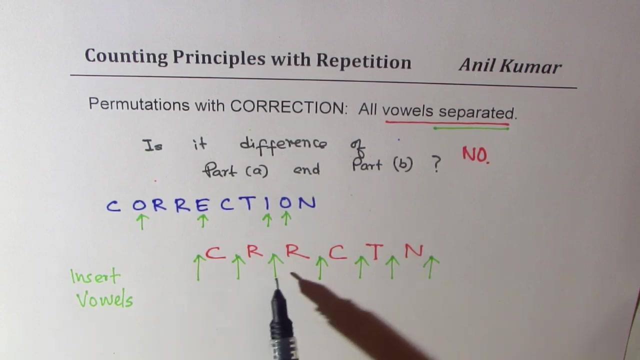 those are different places in which we could insert vowels to ensure they are separated. you are getting the idea right: to ensure that they are separated. these walls could take one of these positions, so they are 1, 2, 3, 4, 5, 6, 7 positions they can take right. 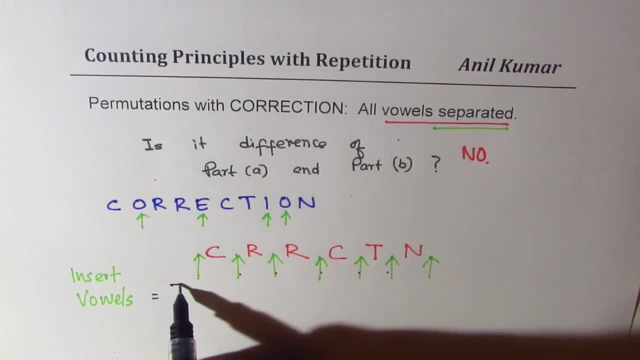 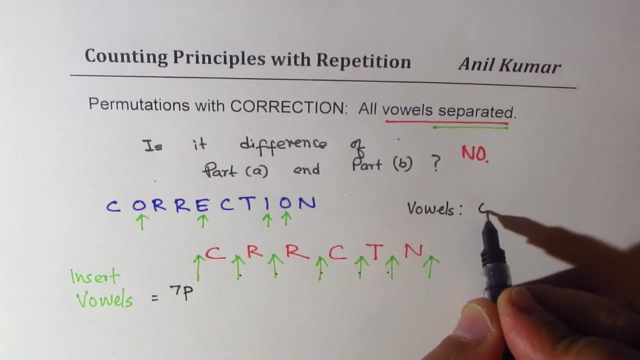 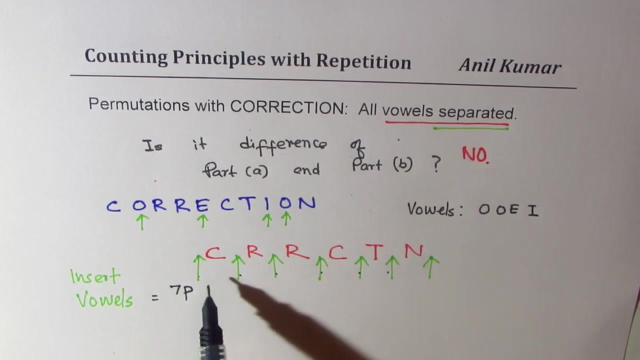 so these positions which they can take are 7, 7 positions they can take, 7 positions they can take, can take. and how many vowels do we have? let me write down again the number of vowels. so vowels which we have are four: two o's, one e and one i. so these are four vowels. so we could actually. 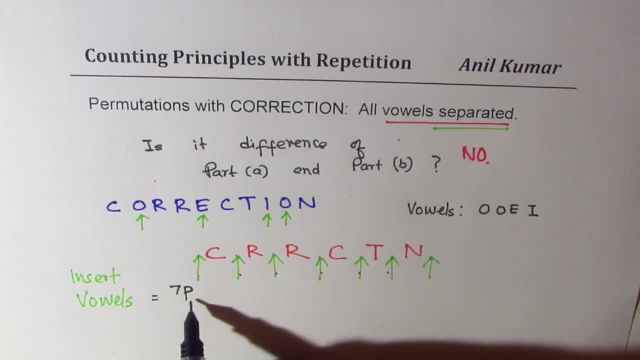 place four of them right seven, p four and out of them two are o's. so we have to divide this by two, factorial, since they are repeated. so that is inserting vowels. you get the idea correct. now let's talk about these placements, that is, placement of consonants. 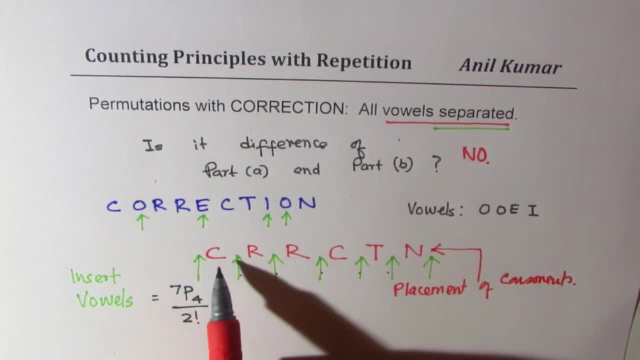 how many of these weren't two, three, four, five, six. so they that will be equal to. let me write down here in a different thing, six factorial, out of which there are two c's, two factorial, two r's, correct, now, if you really want to find total, all vowels separated. now, if you want to find all. 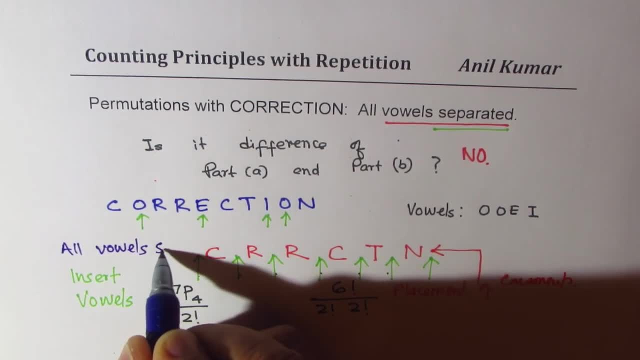 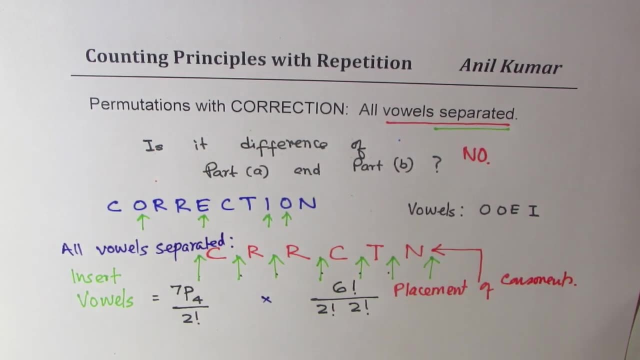 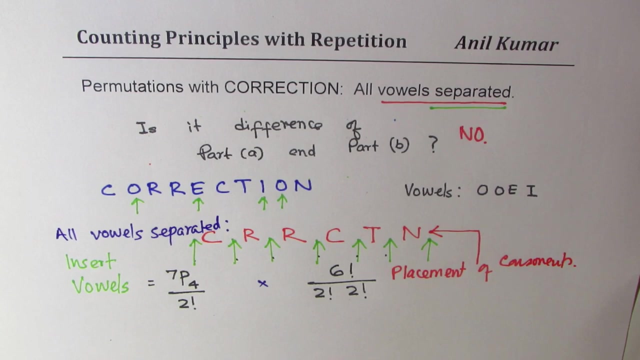 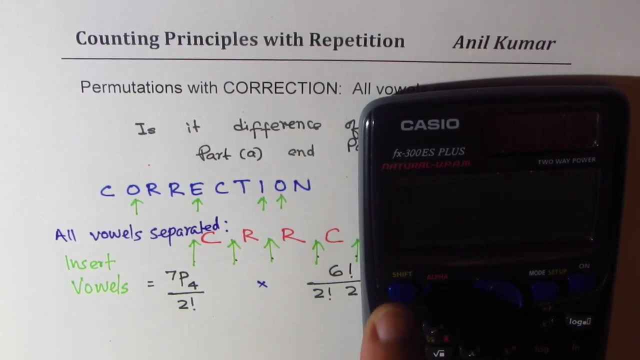 vowels separated, it means it is product of these two. you get an idea. so that is our answer. is that clear, right? so this is, this is the answer for us. so let's calculate this answer using the calculator. so we have 7p4. 7p4, which is equals to 840. 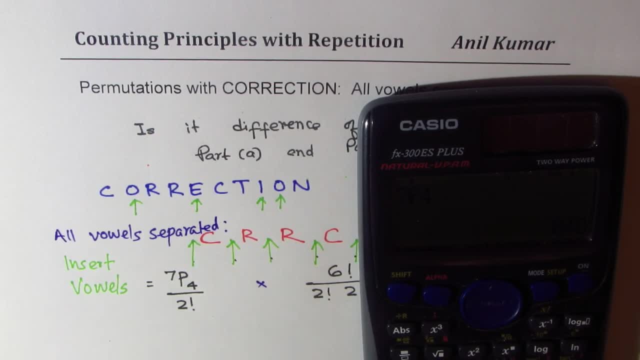 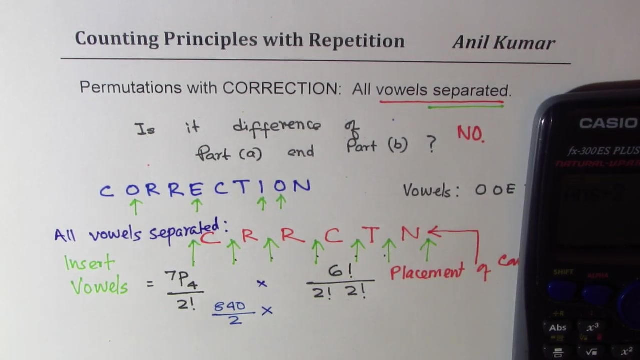 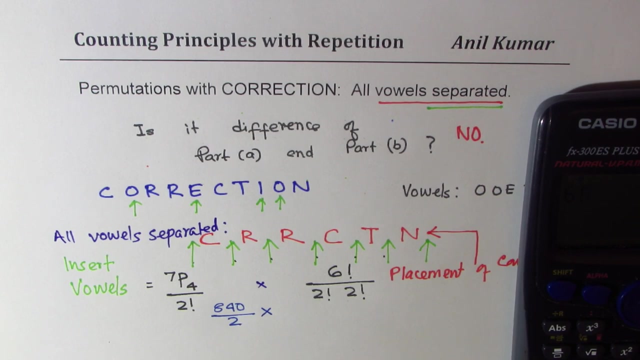 divided by 2. so this is: we get this as 840 divided by 2. so we'll divide this by 2 and then we are going to multiply this by all this, so which is 6 factorial divided by, let's say, 4, 18. 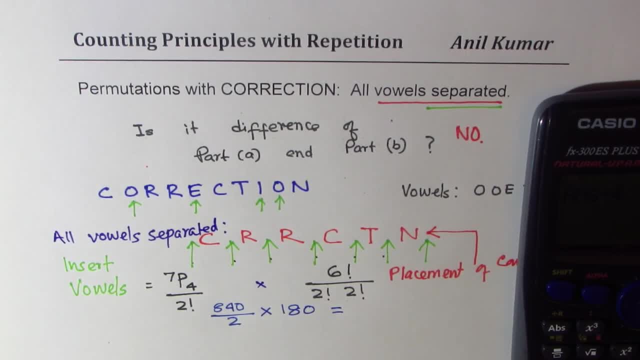 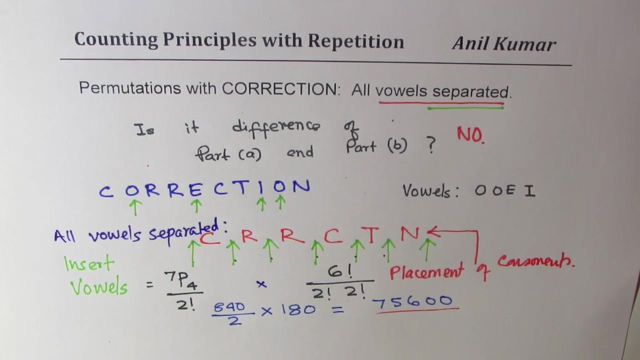 so that is the answer, is it okay? so let's multiply and get the answer. so it is 840 times 180 divided by 2, which is 75 600, right? so the total number of ways is 75 600. that is how we can answer this question. 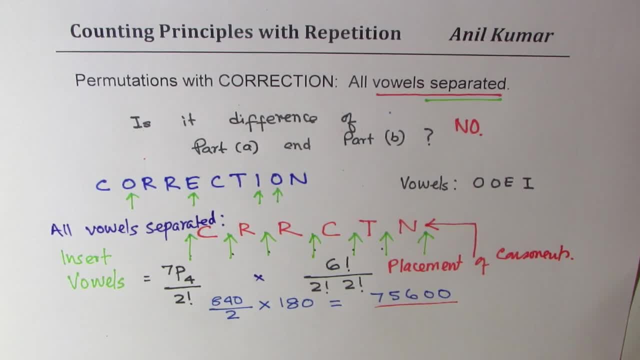 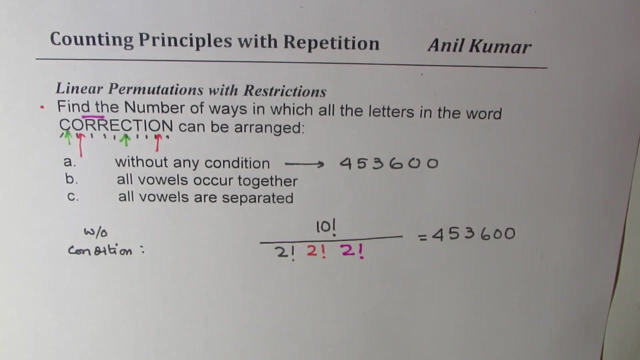 so i hope these steps are useful to you and i hope you have found this video useful to you, are absolutely clear and you also understand what do we mean when we say vowels are together and vowels are separated. right, let's put all the solutions together and see the whole picture.